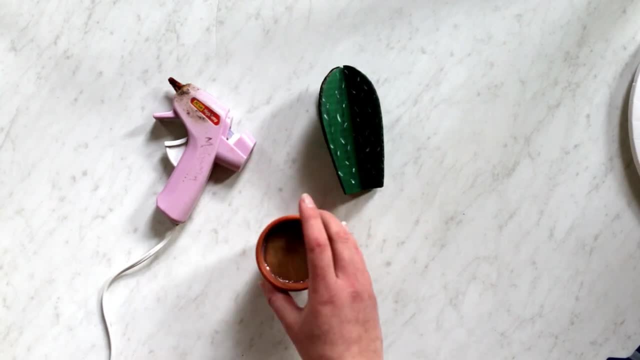 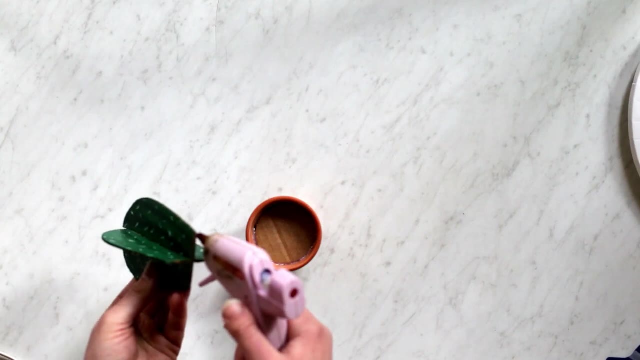 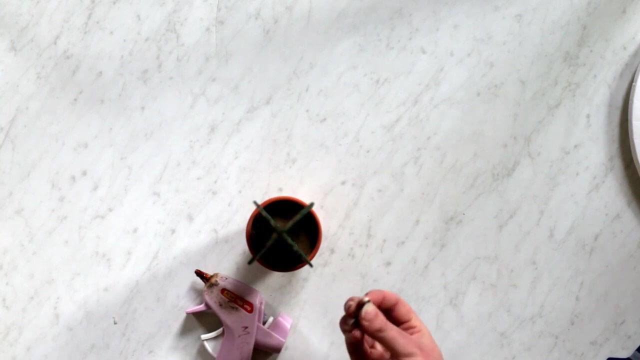 So I glued, um, I put some- there was some soil in this pot- but I put a circular, um, just piece of cardboard, and then I'm just going to glue this bottom piece And then I'm actually just going to put a little bit of extra glue in there and then add a little bit of soil just to make it look like a cactus. 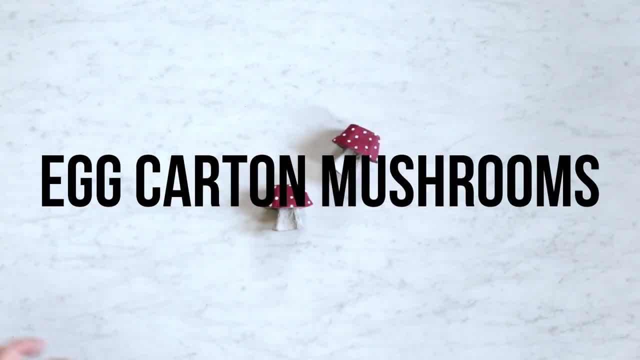 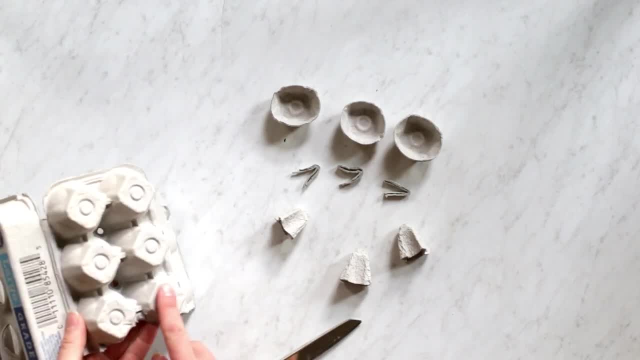 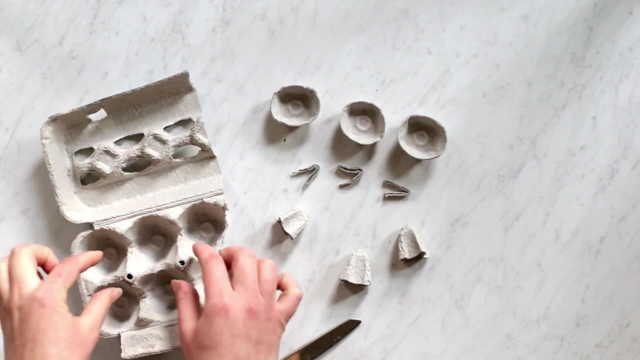 So it's going to look a little bit more real. Okay, So for the mushrooms, I cut the little parts I don't know where the egg set out for the top of the mushrooms, And then I cut out these things in between the eggs for the base. 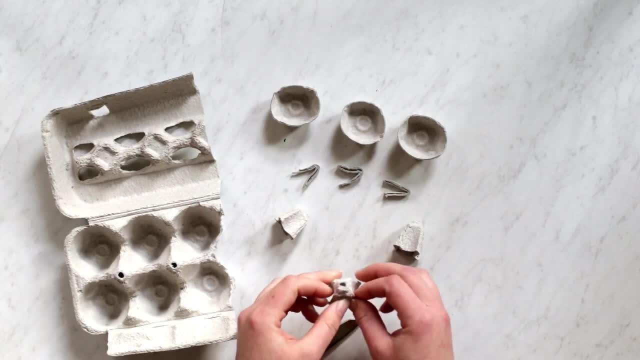 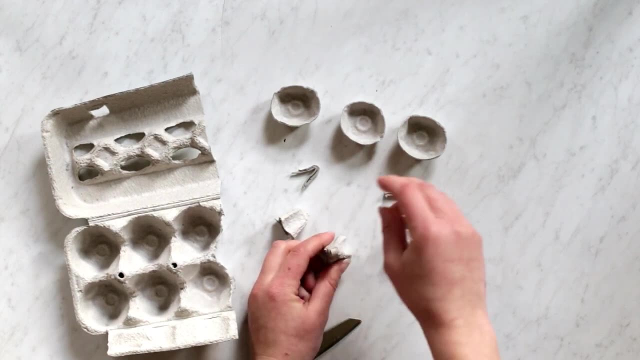 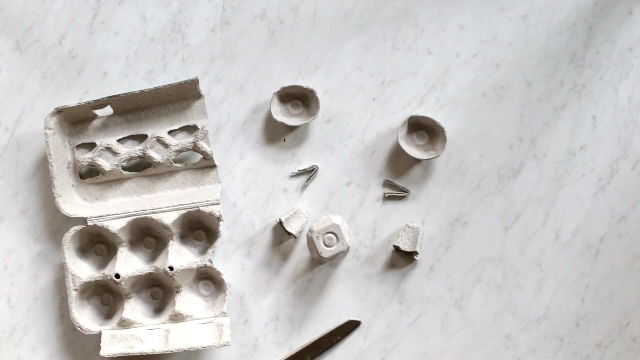 And so for each of the bases I just kind of squeezed them together to make it a little bit more narrow, And then I just used a scrap piece to stick down into here Just to make it a little bit higher once I glue the top of the gusset line. 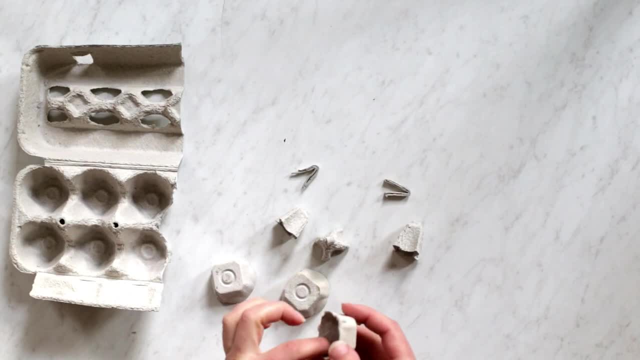 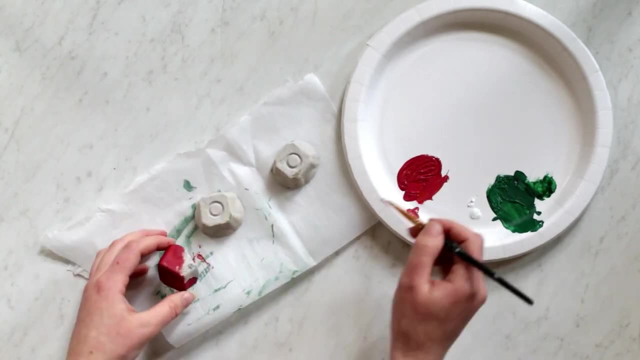 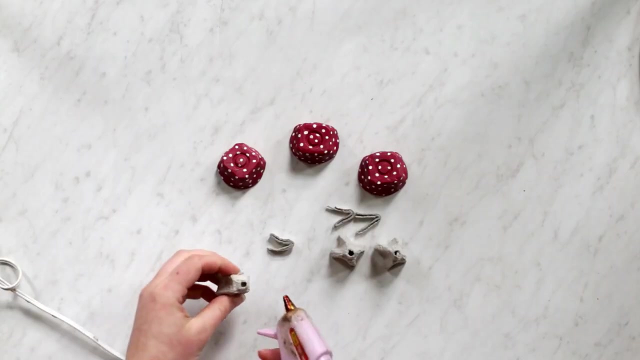 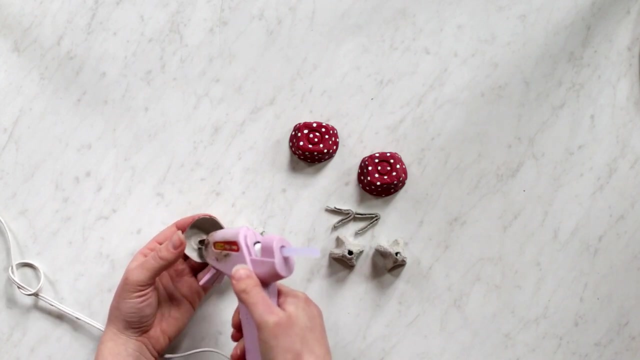 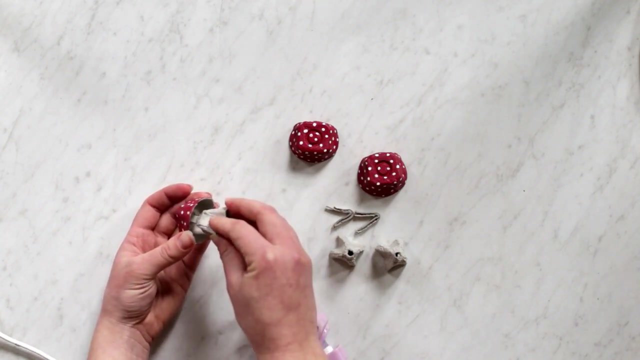 So now I'm just going to paint the tops red and then put little dots on them, and then I'll glue everything together. Now I'm just going to glue the tab in place and then on the inside of the mushroom cap I'm just going to put some glue and then stick it onto the extra piece. 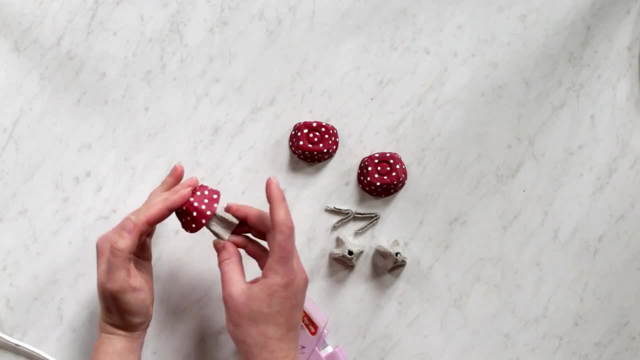 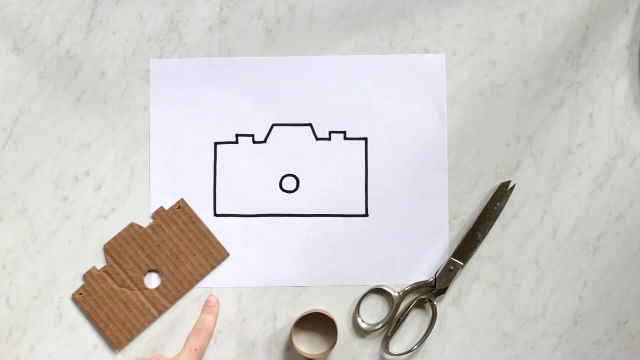 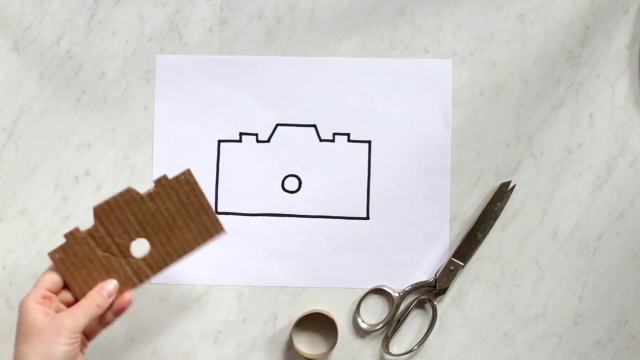 There we go. So for the camera, I actually did two different styles. So the first one: you can just use this printable of a PDF I'll include on the blog and then just trace it onto cardboard and cut it out, and then I put two little holes on the side. 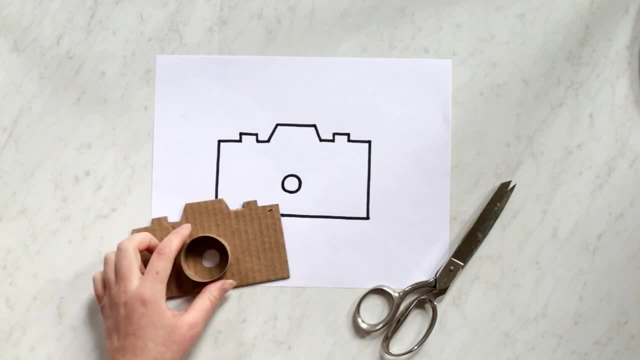 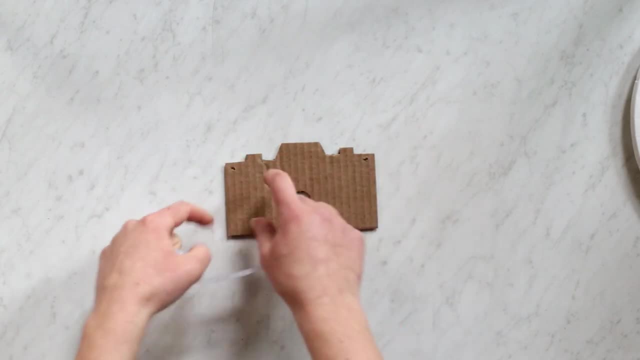 so I can put string through, and then I'll just glue this in place and then I'm just going to paint everything. So I'm just going to use washi tape and I'll just stick it on. There we go, Just stretch it across so I can get a black strip across the camera, and then I'm also. 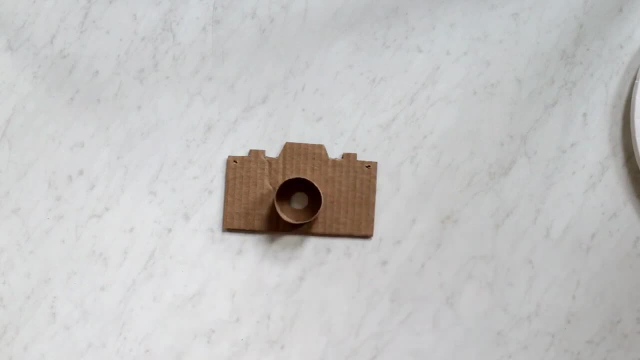 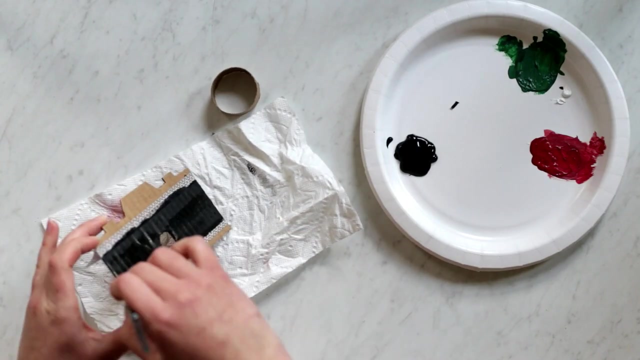 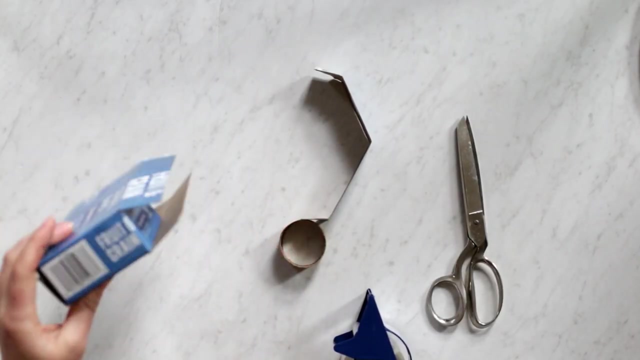 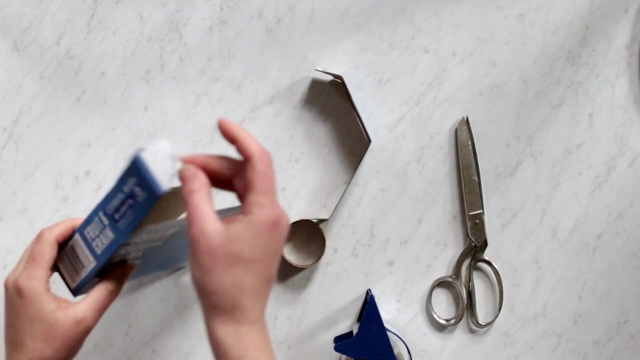 going to paint the piece of the cardboard tube that I cut black as well. And then for the second camera I took just like a thin box from cereal bars and I cut it down. So from the top I cut just like an inch, a little over an inch off the top and left. 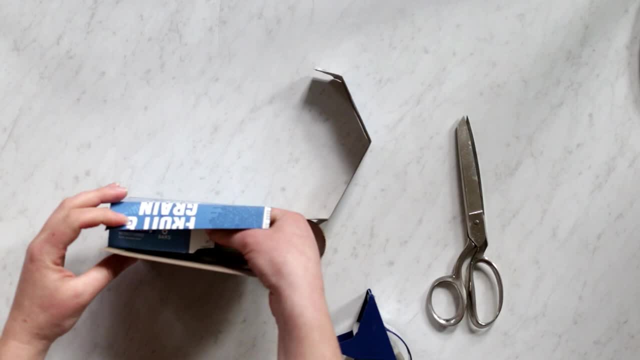 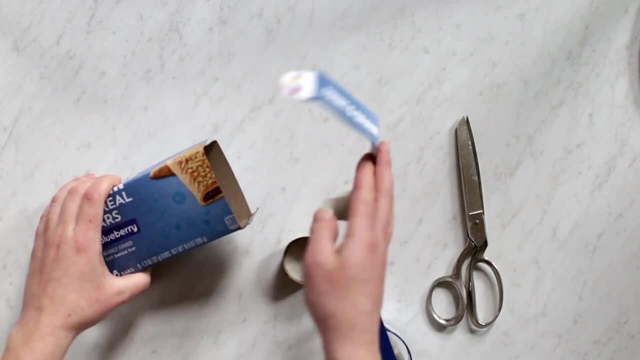 the side flat and then I folded that down in and then I'm going to fold the top two sides. I just bent it along and then this part of the box I had to cut off. so I cut off the opposite end and I'm just going to tape that inside. 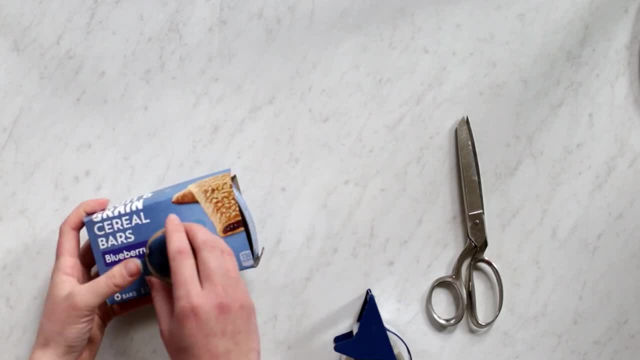 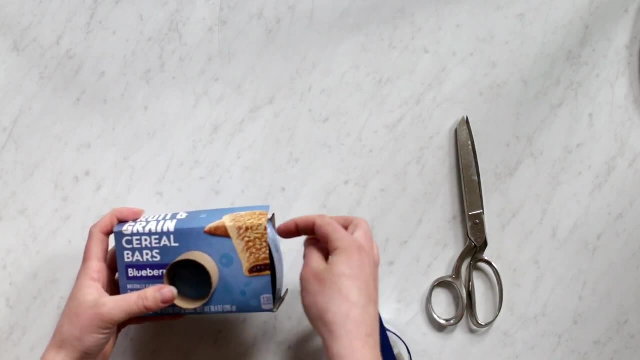 So now I'm just going to tape the whole box together pretty much, and then I'll glue this on the front. I'm going to glue some little extra pieces on and I'm just going to poke holes before I tape it all together for string to go around and then for a little hole from the back to 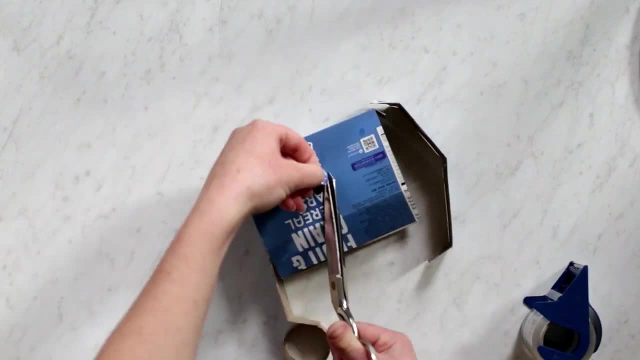 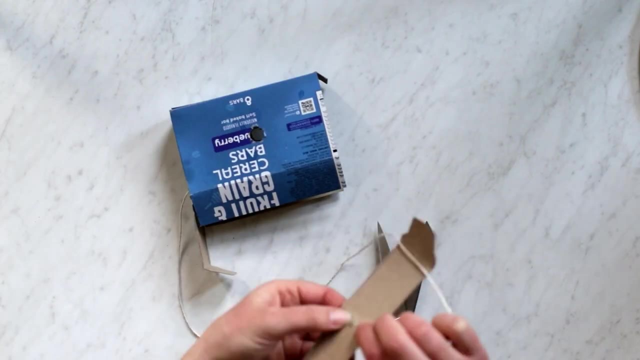 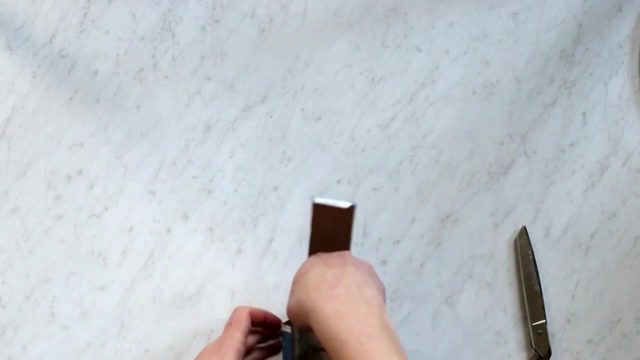 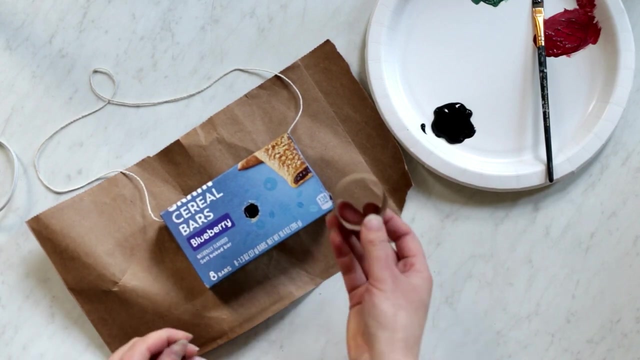 the front. So I'm just going to put the string through the sides and now I'm just going to tape everything together. Okay, Okay, Okay, Okay. And now I'm just going to paint the whole outside of the box black and this piece, and 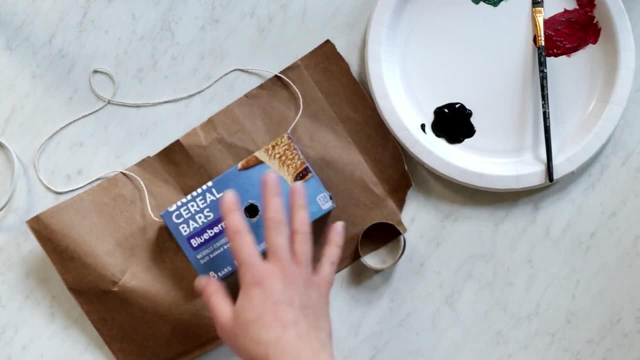 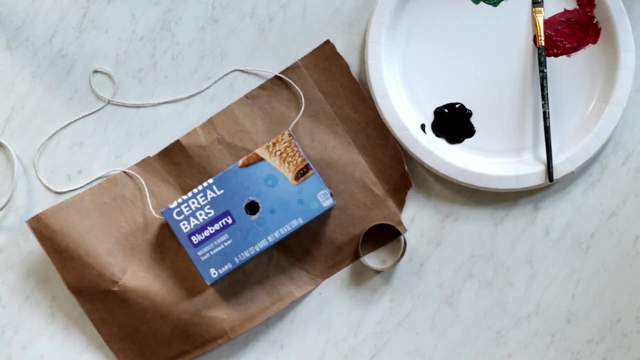 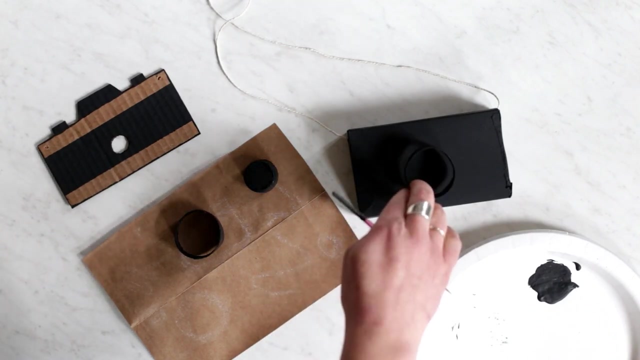 I'm going to go get a couple pieces to put on the sides or on the top for the buttons, just like a couple caps from pop bottles and stuff, and I'll paint those black as well and then I'll paint a design onto it later. Now I'm going to paint some extra details on the other parts of the camera and then 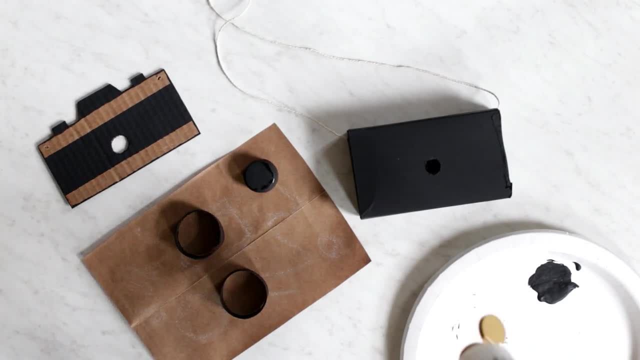 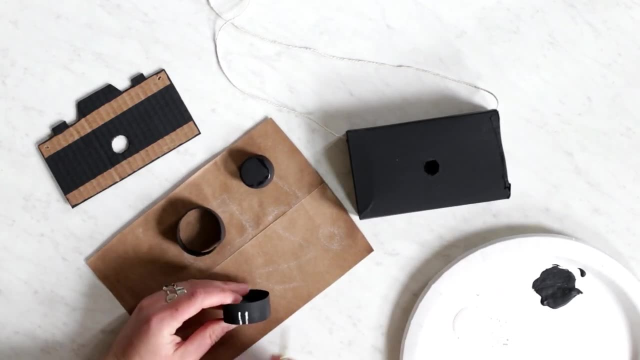 a couple different things on the camera to give it a little more realistic. look Okay, Okay, Okay, Okay, Okay. But you can have your kids paint it however they want, And now I'm just going to use a hot glue gun to glue everything in place. 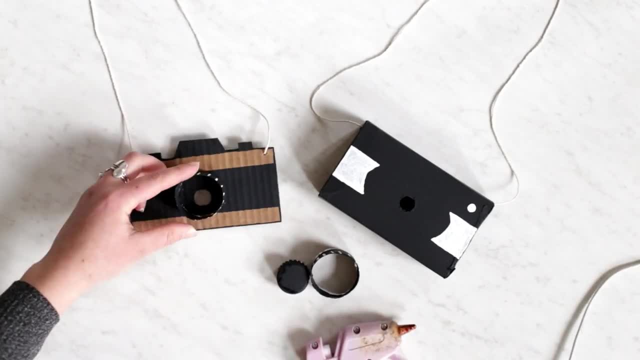 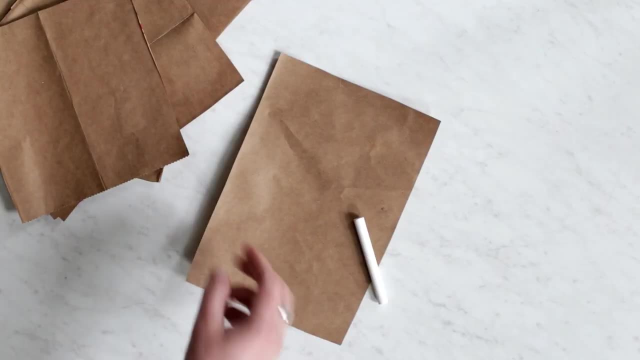 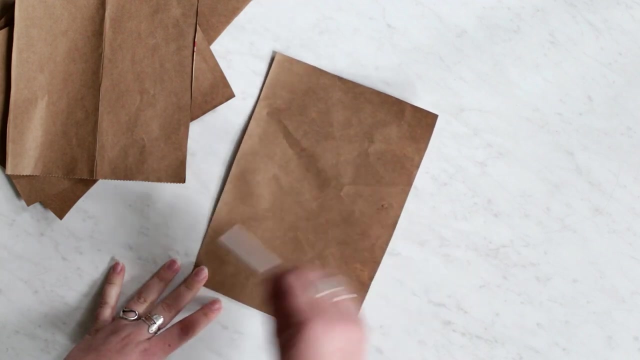 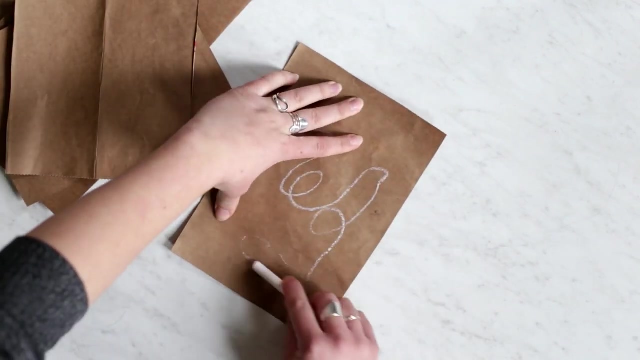 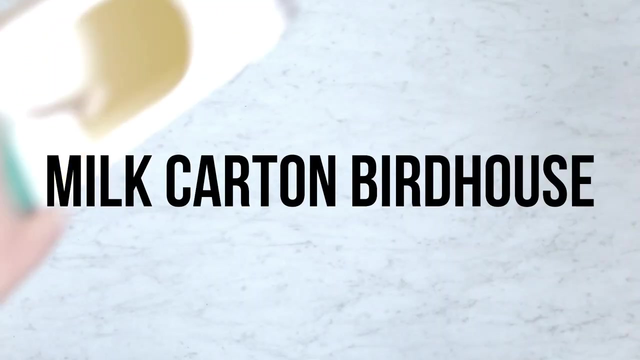 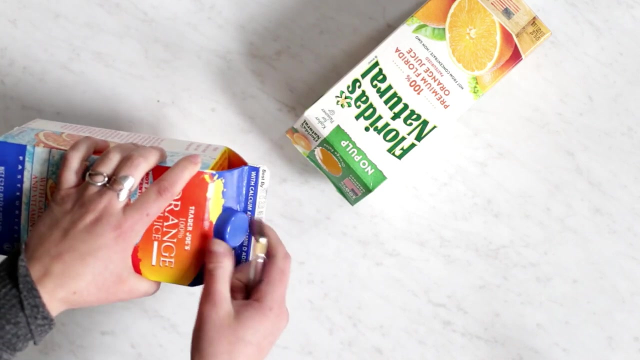 You're just going to cut out pieces of paper bag and then you're just going to give your kid some chalk- Okay, draw doodles on there, and then you can just frame it, this little abstract art. so first I just took my x-acto knife and then I cut around the cap and then I cut. 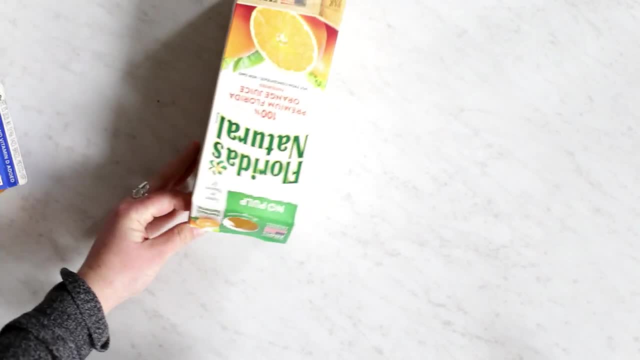 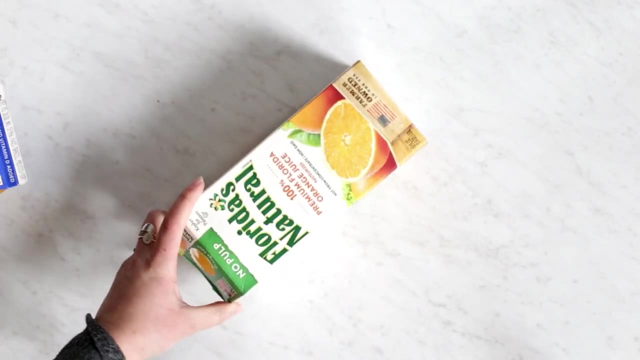 the top part off, so that it ended up looking like this, and then you can just give it to your kid to paint, or I'm actually just gonna spray paint the first coat and then paint on top of it, just to make it a little bit easier. so 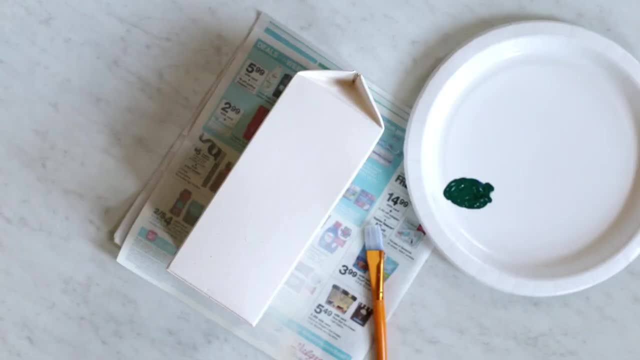 I'm gonna go take it, spray paint it and then I'll paint it afterwards, and then, once you have the base coat all set, you can just use a bunch of different color paints, paint it however you want, have your kids paint it however you want, and then let it dry. so then I just cut out a square, which I'll include in the PDF, and 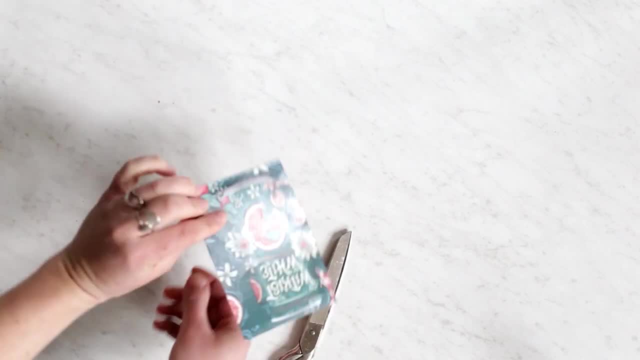 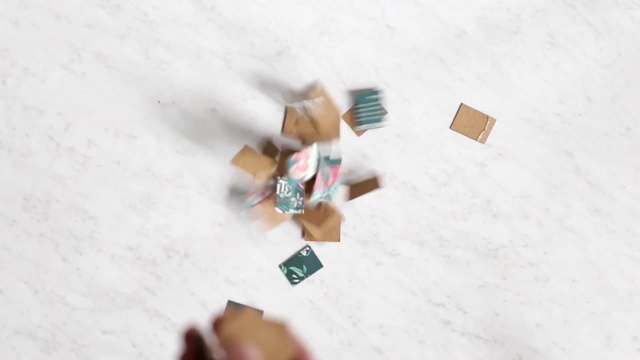 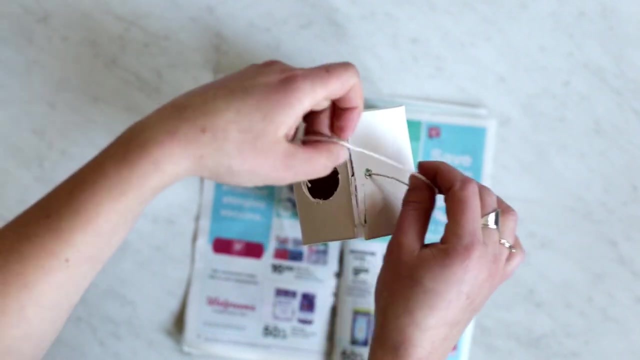 then I'm just gonna cut a bunch of the tiles out of just a piece of cardboard and then I'm going to use those as the rake. then I'm just going to take some string and tie it. I just cut a little hole on the side and then through the spot where you normally would pour it, and this is. 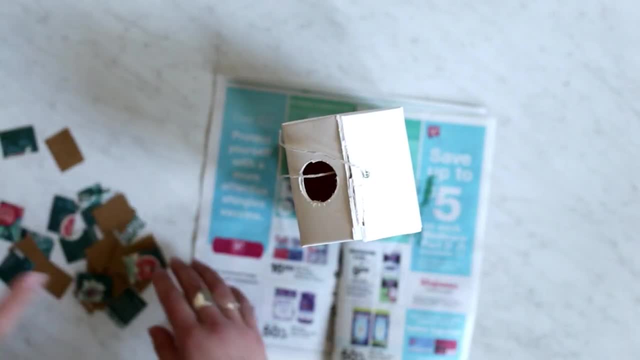 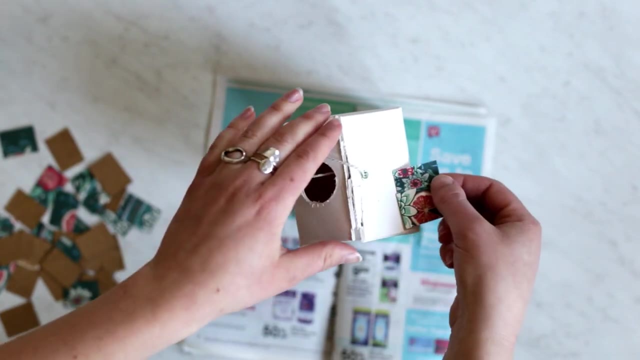 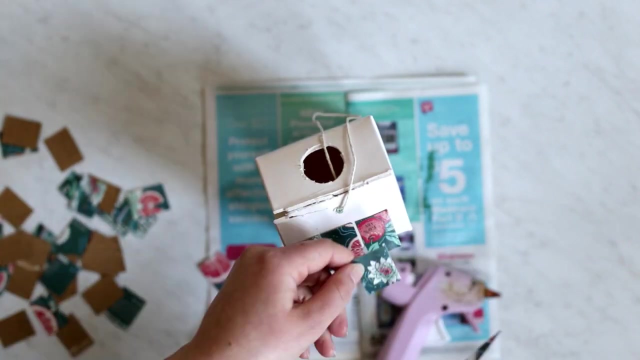 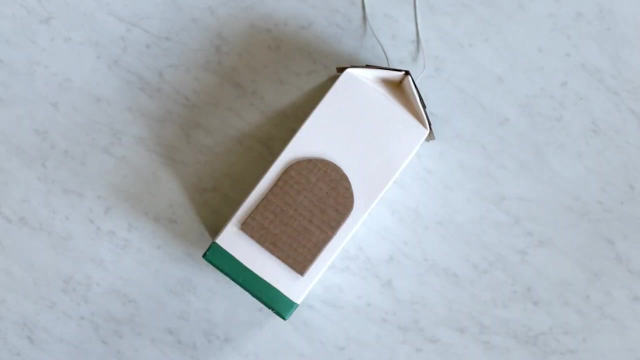 just gonna serve to hang it up, and then I'm gonna start taking these pieces that I cut and I actually really like the color of the box, so I'm gonna start creating like shingles and then hot gluing them in place on top. now I'm just gonna use the arch from the printable and I'm just gonna trace it. 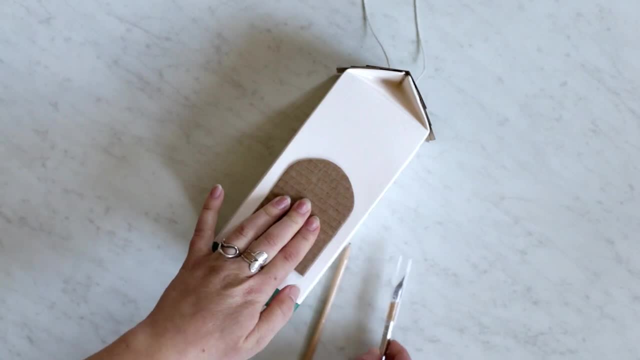 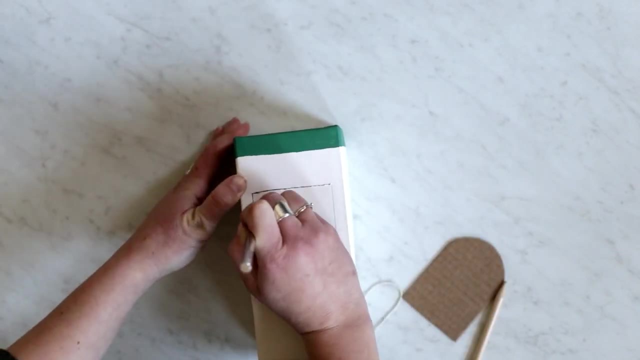 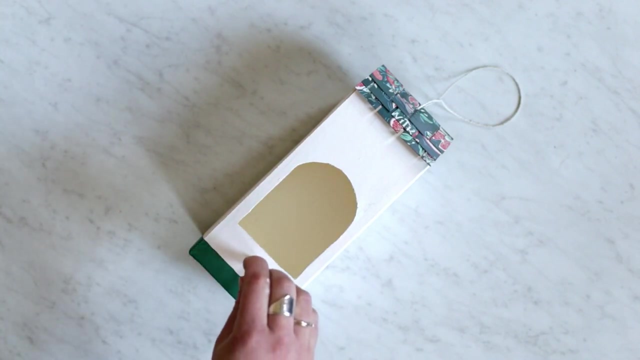 onto the side of the box and then I'll use an exacto knife to cut it out. so now I'm just gonna cut a small hole under here and then I just have this like piece of a wooden doll and I'm gonna glue it in place. 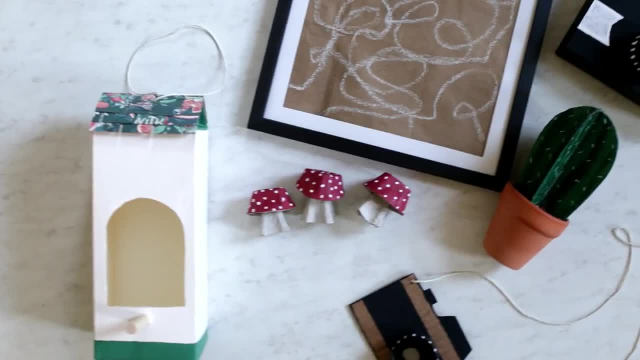 and then I'm just gonna cut it out, and then I'm just gonna trace it onto the other side of the box.